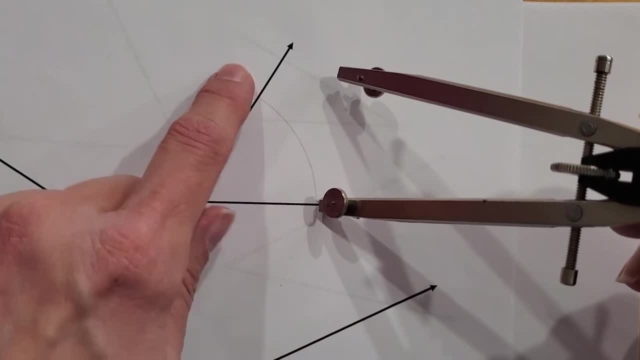 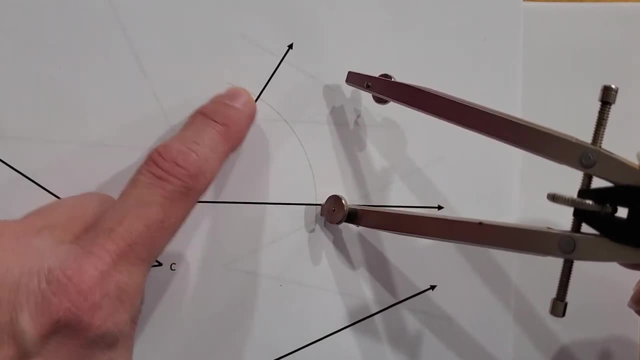 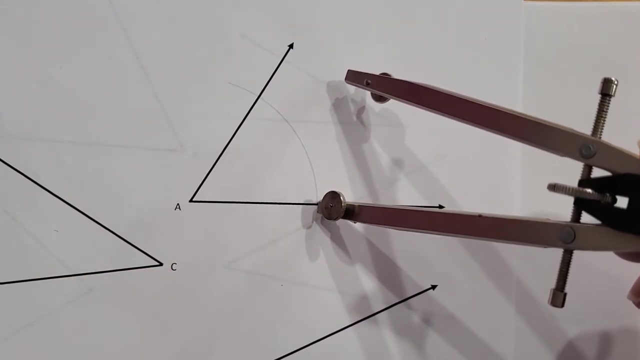 want to make an arc, that with the center, on each of the arcs that intersected the sides of the angle. So one time with the center here, the next time with the center there, We're going to draw an arc in between the angle, So, and I'm going to have to keep the radius the same. So for this one, 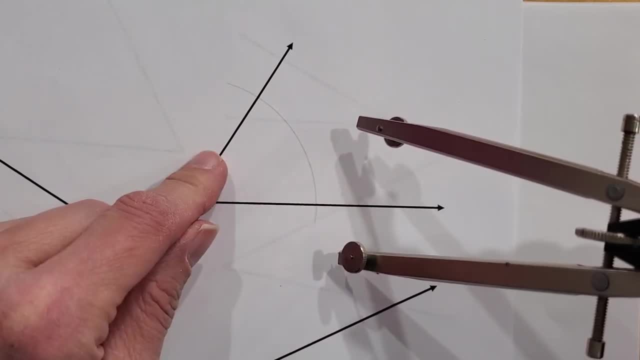 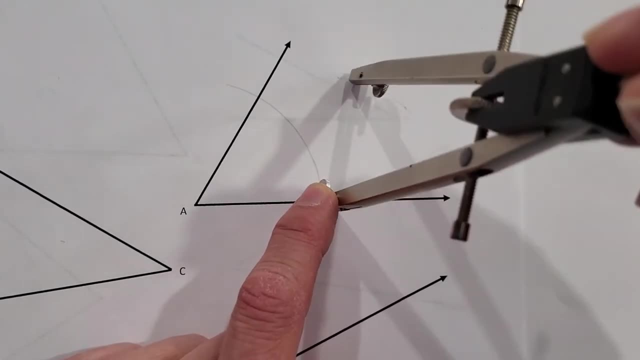 you can change it from the first step to the second step, but from the second step to the third step you cannot change your radius. Those are some of the things I'll check when I grade your work. So I'm going to make an arc right there, Try to make it a little darker And then 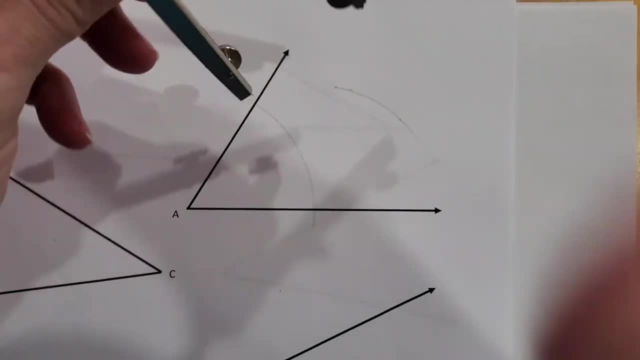 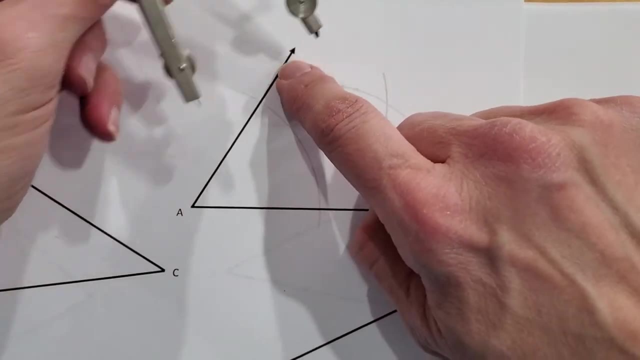 I'm going to do the same thing without changing my radius. I'm going to do the same thing over here, Knocking my phone over, Okay, So remember, I didn't change the radius. That means the distance from this arc to where those two 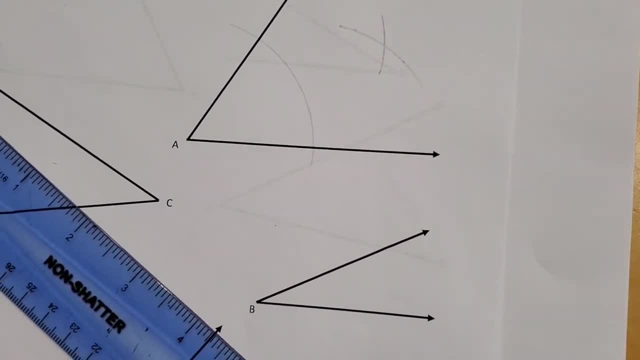 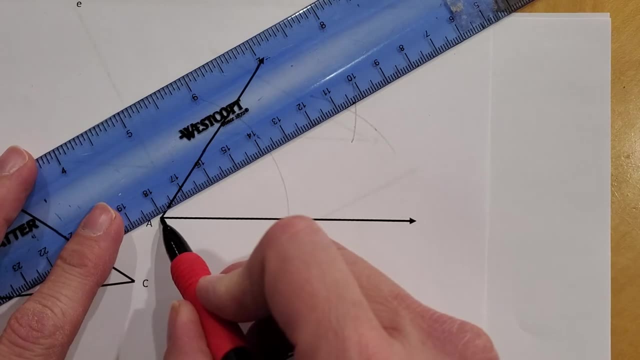 arcs intersect and from this arc to where those two intersects are exactly the same. That's why it's an angle bisector, because I'm actually finding the point in the middle of the angle. I know this vertex is in the middle of the angle. I know now that that point is in the middle of. 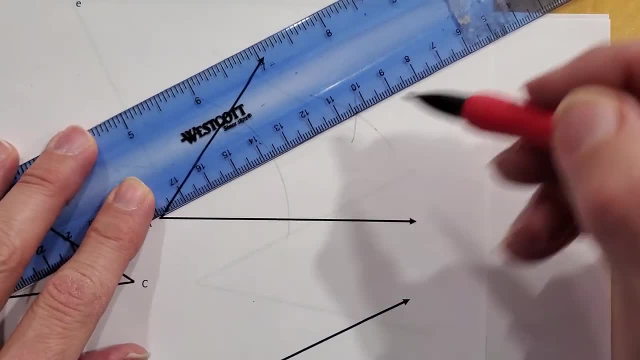 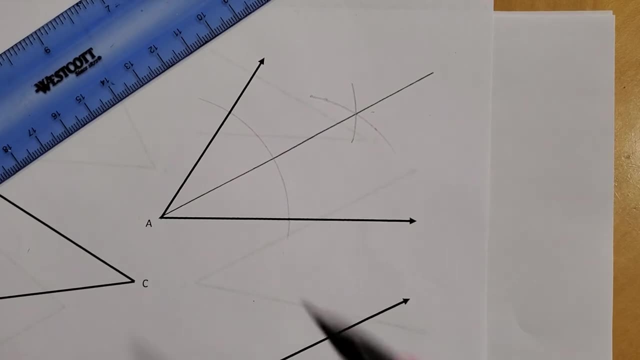 the angle. If I draw a line between the vertex and the point that's also in the middle of an angle, I get a line that holds all the points that are smack dab in the middle of the angle. So that means these. now, these two little parts are the same, because an angle bisector divides an angle into two. 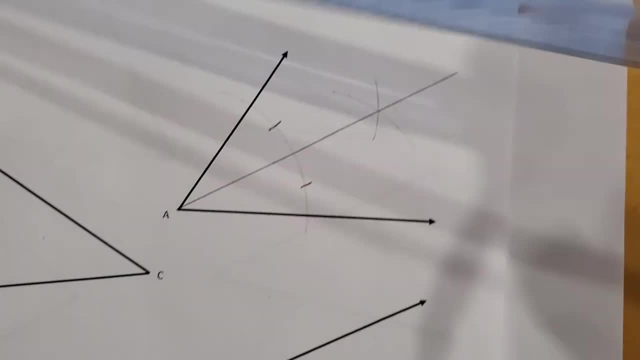 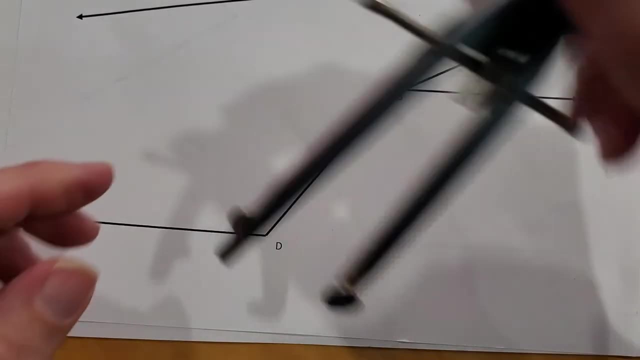 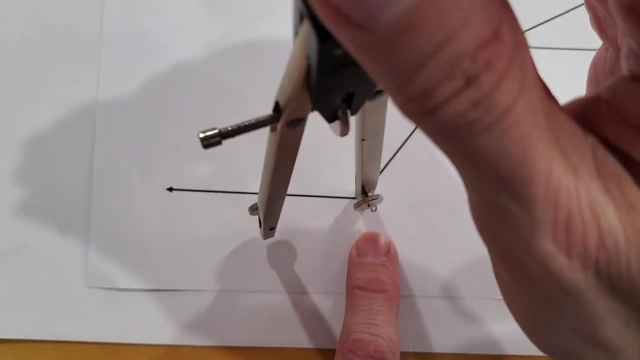 congruent parts. Let's do that one more time. I'm going to do it on an obtuse angle, because sometimes that can be a little tricky for some people. So again, I'm going to just use a convenient radius. So I'm going to put the center of my compass at the vertex and I'm going to make an 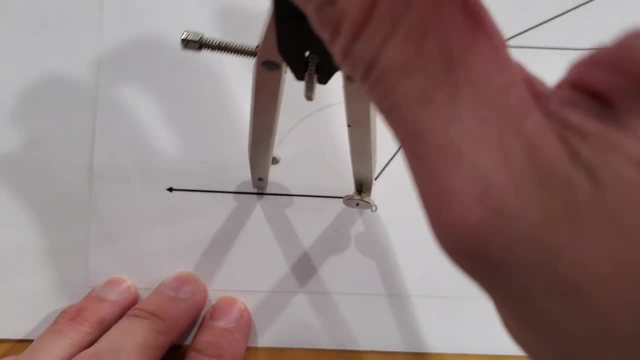 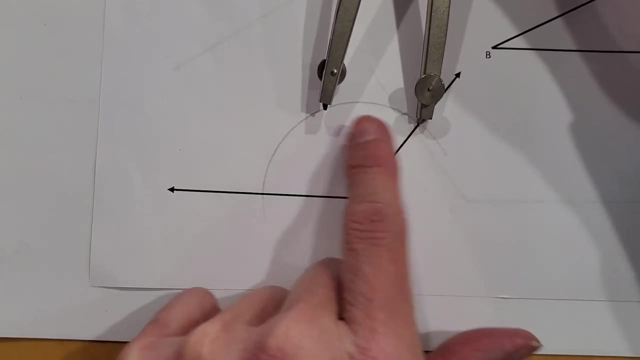 arc that intersects both sides. That's got to go way, way around for the obtuse angle. Now, this time, as you can see, I'm going to have to make my arc bigger, because if I'd made an arc in the middle it wouldn't intersect the other one. So you want. 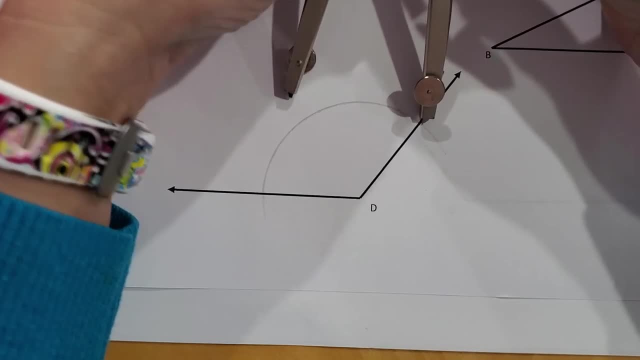 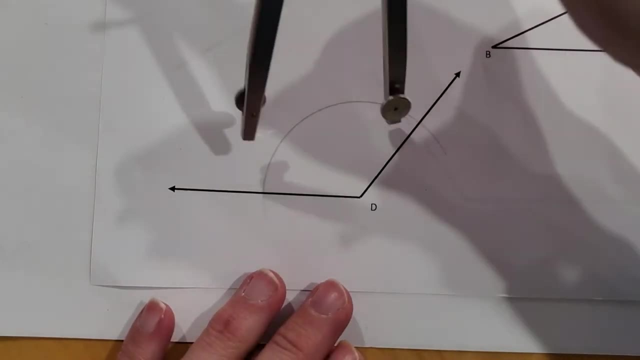 that distance to be more than half the distance that it's going to be to the center of the angle. So just keep that in mind. Sometimes that's tricky with an obtuse bisected angle, because you forget and then you have to redo it. So just heads up on that. So I'm going to draw my arc.